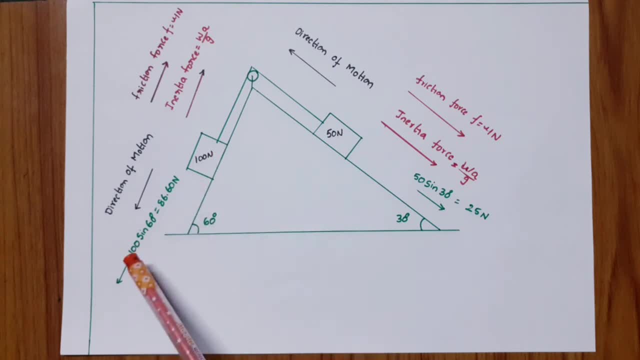 The direction of motion is towards 100 N. So for 100 N block, the block is moving downwards, So the direction of motion is downwards, The inertia force and friction force acting upwards. So for 50 N, the direction of motion is upwards. 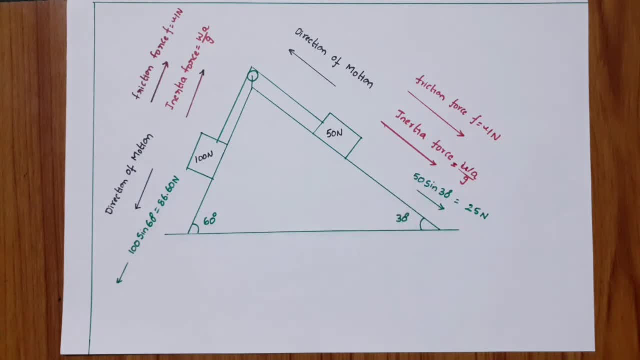 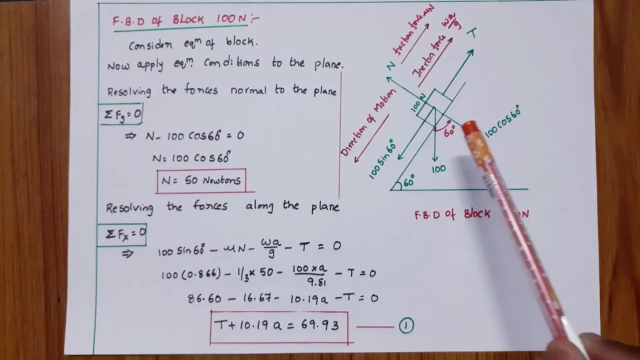 The friction force and inertia force acting downwards. The friction force and inertia forces are the resisting forces, So these forces are acting always opposite to the direction of motion. Now, FBD of black 100 N. So this one is the black 100 N. 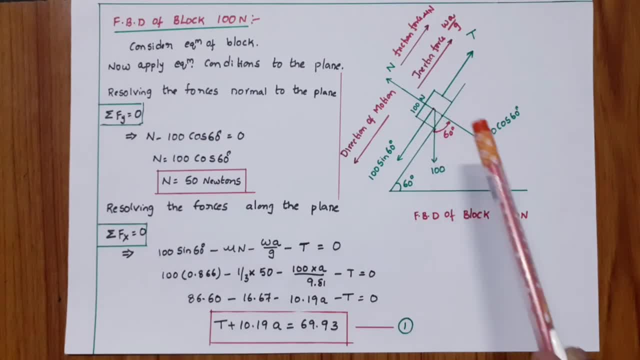 So here the contact between the plane and the black, a normal reaction is generated. So here the weight of the black: 100 N acting downwards. The component normal to the plane is 100 cos 60.. The component along the plane is 100 sine 60.. 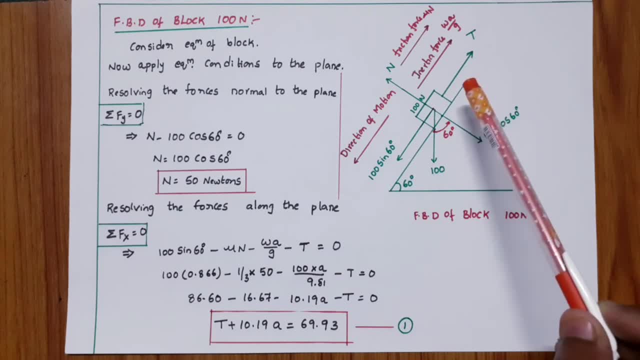 So here this one is the string. The tension of the string is always acting away from the block, So the tension of the string acting upwards. So here the direction of motion is downwards, The friction force and inertia force acting upwards. 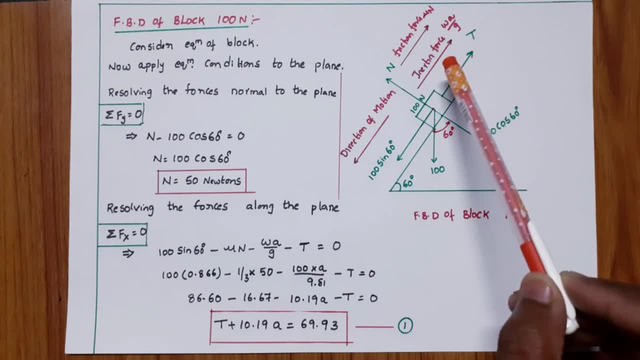 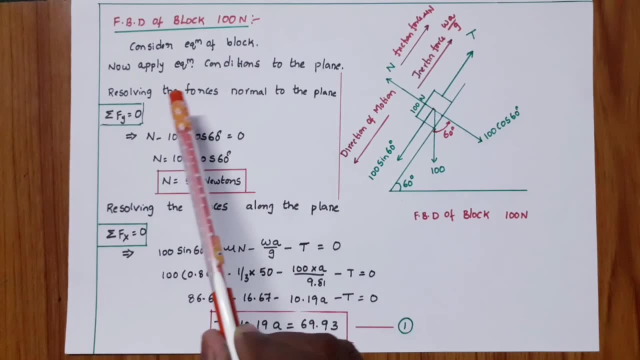 The friction force and inertia force are acting always opposite to the direction of motion. Now consider equilibrium of the block. So now apply the equilibrium conditions to the plane. Now resolving the forces normal to the plane. So now sigma F equal to 0.. 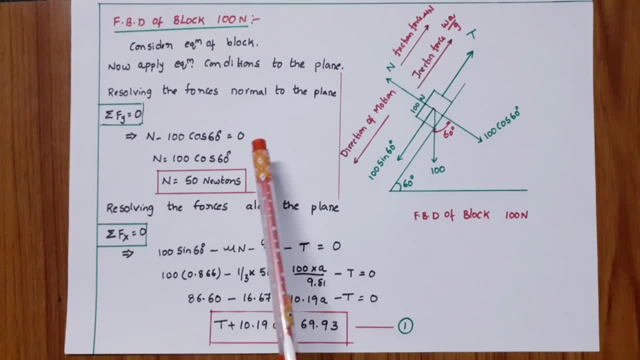 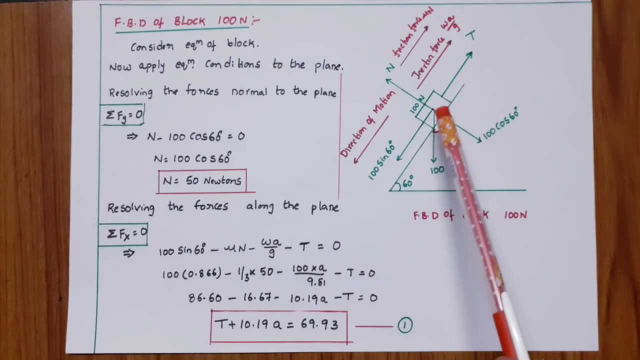 So what is sigma F equal to 0? The sum of the forces in vertical direction is 0.. So what are the forces acting normal to the plane? N and 100 cos 60.. N acting upwards and 100 cos 60 acting downwards. 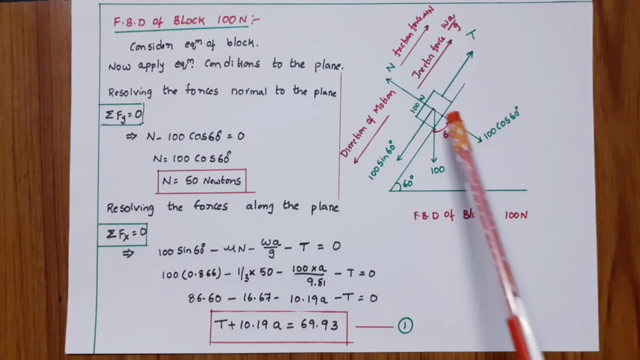 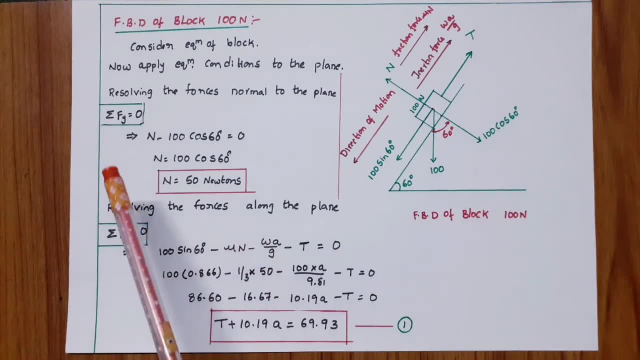 The force which is acting upwards is positive, The force which is acting downwards is negative. So normal reaction: N is positive And 100 cos 60 is negative. So N minus 100 cos 60 is equal to 0.. So N equal to 100 cos 60. 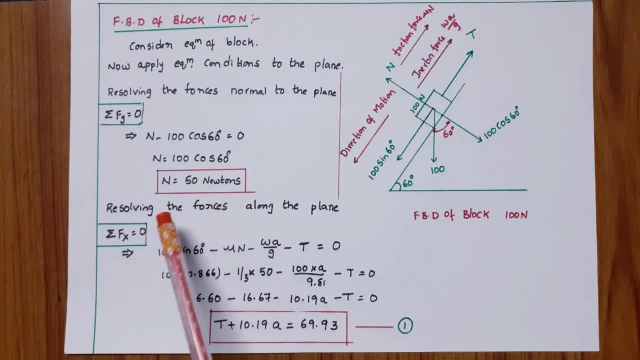 So what is cos 60?? 1 by 2.. So N equal to 50 Newtons. Now resolving the forces along the plane, So sigma F equal to 0.. The sum of the forces in horizontal direction is 0.. 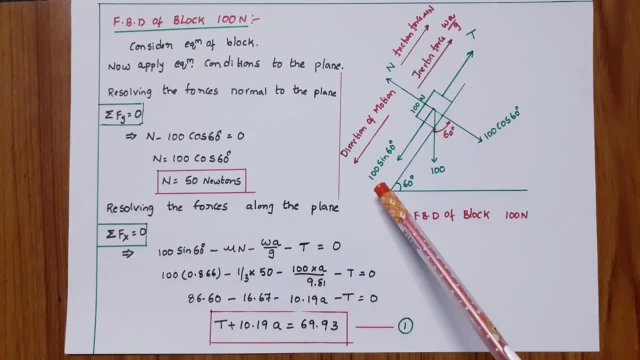 So what are the forces along the plane? 100 sin 60 tension force, inertia force and friction force Are acting along the plane. So now, what is the force in direction of motion? 100 sin 60 is the force in direction of motion. 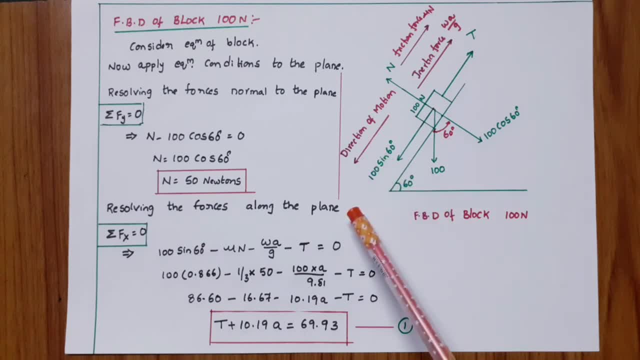 So it is positive: Friction force, inertia force and tension force acting opposite to the direction of motion. So all these forces are negative forces. 100 sin 60 minus friction force, minus inertia force, minus tension force is equal to 0.. 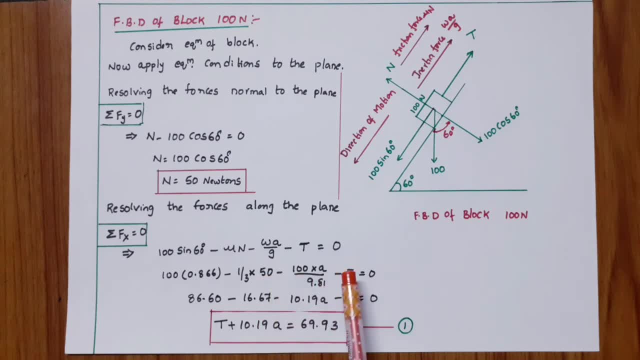 100. sin 60 minus mu N, minus W by Z, minus tension force, is equal to 0.. mu N minus W by Z minus T, equal to 0.. So 100 into So what is sin? 60? 0.866.. 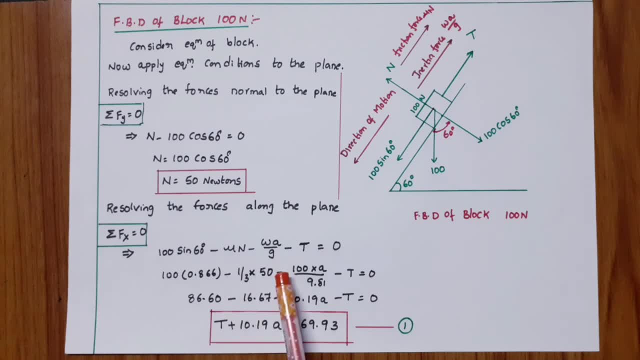 mu is 1 by 3.. N is 50.. So W by Z, What is W? 100.. Z is 9.81 into A minus T equal to 0.. So 86.60 minus 16.67 minus 10.19, A minus T equal to 0.. 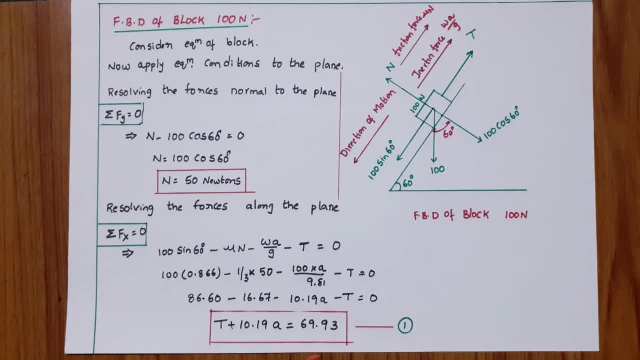 T plus 10.19 A minus T, equal to 0.. T plus 10.19 A minus T, equal to 0.. T plus 10.19 A minus A is equal to 69.93, so this equation is number one. 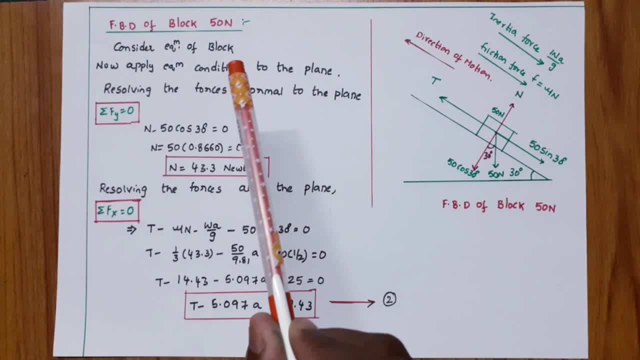 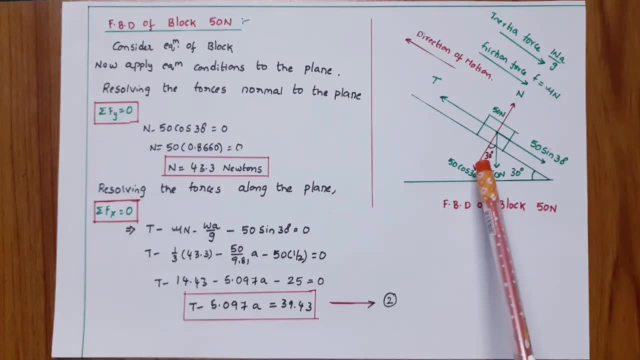 Now weight of Ramopyra net, So 1. FBD of tan, FBD of whiteius black: 50 N, 15 N. So here the contact between T and Whiteius Yellow rainbow propos yard is normal, reaction is generated. 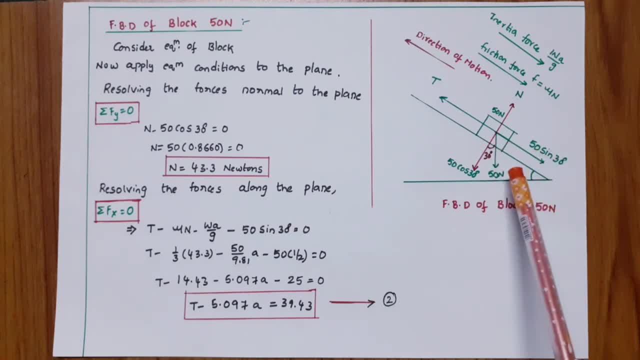 So here, weight of Black moving Nuclear reaction down towards 50N component of Whiteius Yellow rainbow. Integration of Whiteius Yellow and Black is 50 Sans 30. The component along the plane is 50 Sin30. 30 degree. so here this one is the string. the tension force is acting always away. 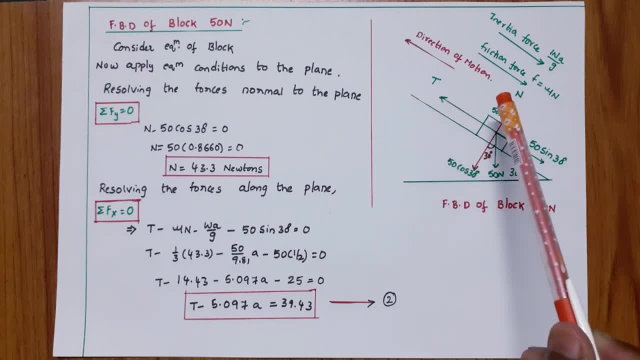 from the block. so the tension is acting upwards. so now the direction of motion is upwards, the inertia force and friction force acting downwards. the inertia force and friction force are acting always opposite to the direction of motion. so consider: equilibrium of the block. now apply the equilibrium conditions to the plane. so now resolving the force is normal to the plane now. 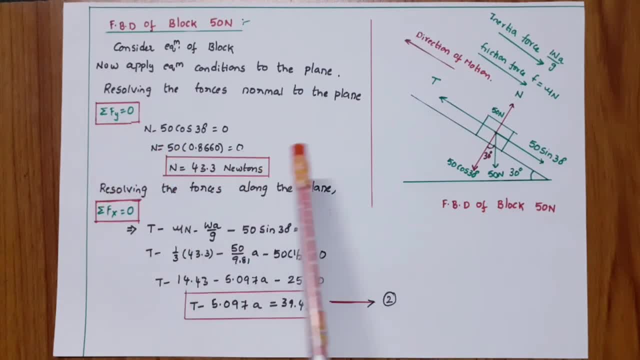 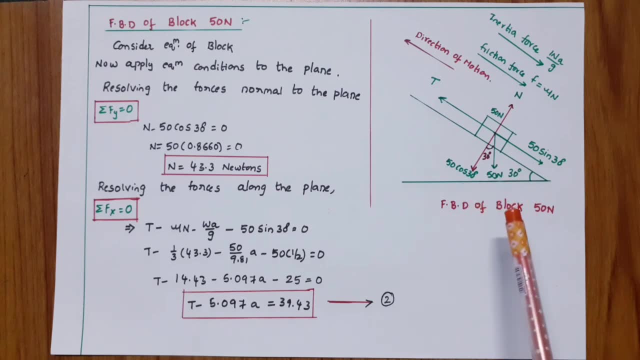 Sigma f equal to zero. the sum of the forces in vertical direction is zero. now what are the forces? normal to the plane, normal reaction and 50 cos 30 degree. the upward force is positive and here the downward force is negative. so n is positive and 50 cos 30 is negative. n minus 50 cos 30 degree, equal to zero, n. 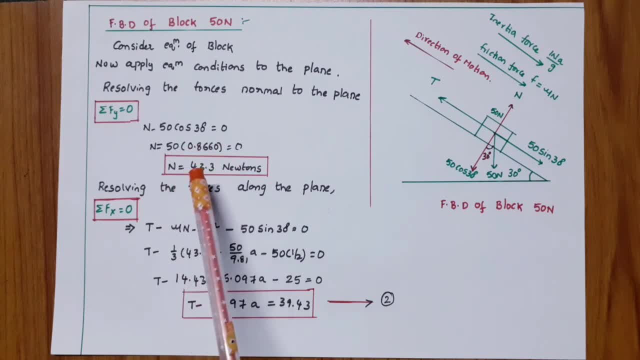 equal to 50 into what is cos 30. 0.8660 is equal to zero, n equal to 43.3 newtons. so now dissolving the forces along the plane. what are the forces along the plane? tension force, comma, friction force, common inertia force and 50 sine 30. 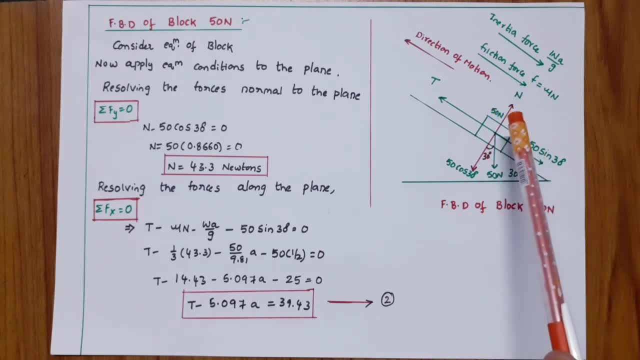 degree the forces which are acting in the direction of motion is positive. so what is the force acting in direction of motion? so tension is the force in direction of motion. so tension is positive and all the remaining forces are negative. so tension force minus friction, force minus inertia. 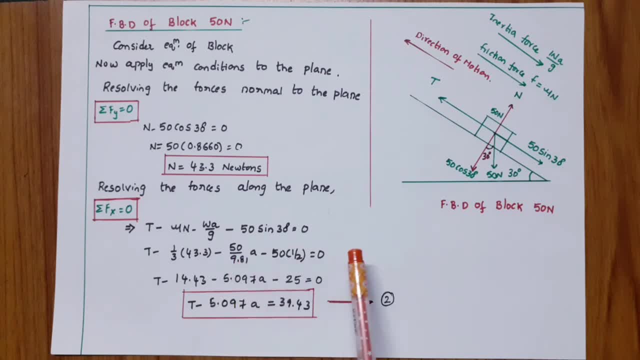 force minus 50, sine 30 degree equal to 0. so t minus what is mu? 1 by 3, n is 43.3, so w by z, w is 50, g is 9.81 minus 50 into sine 30, so what is sine 30? 1 by 2 equal to 0. 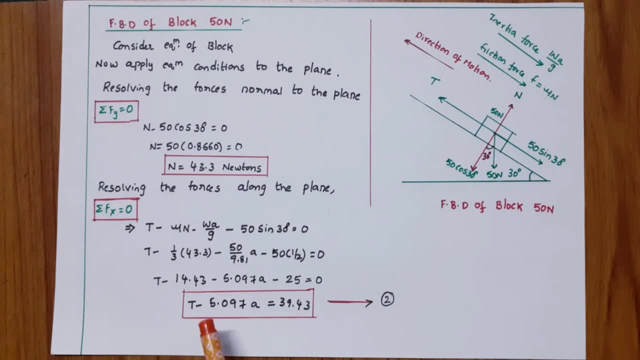 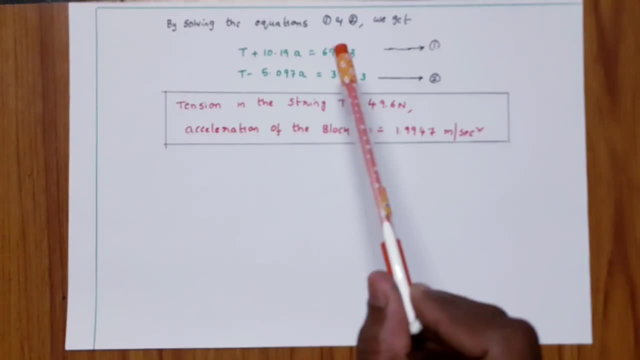 so t minus 14.43. so minus 5.097 a minus 25 equal to 0. so t minus 5.097 a is equal to 39.43. this one is the equation number two. by solving the equations one and two comma, we get: 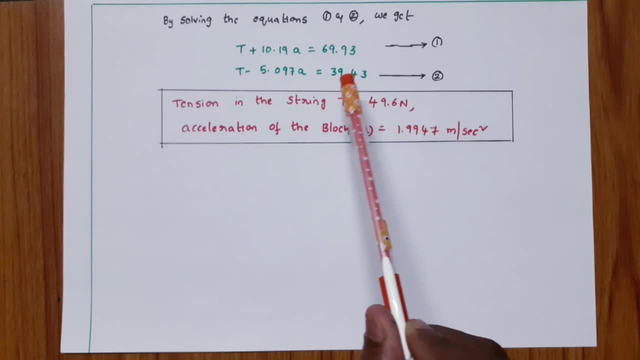 so t plus 10.19 a equal to 69.93. t minus 5.097 a is equal to 39.43. three. this one is the equation number two. so by solving these two equations- tension in the string t, equal to 49.6 newtons, and acceleration of the block, a equal to- 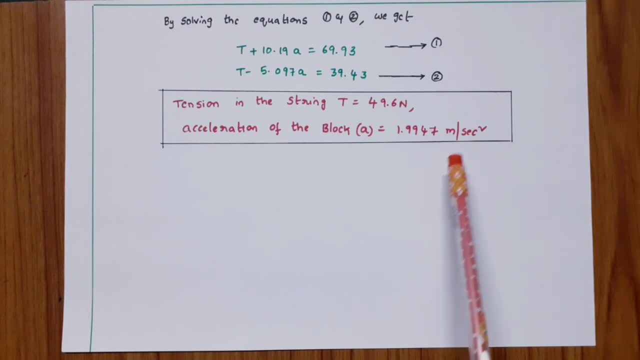 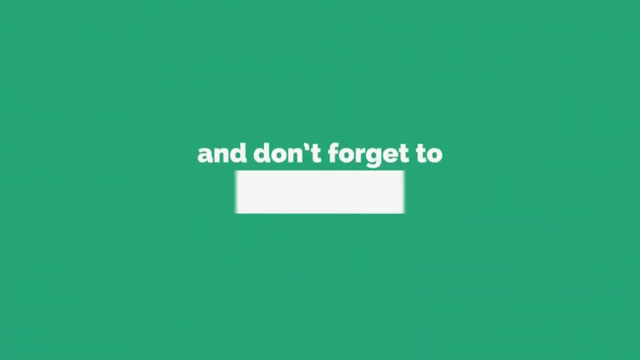 1.9947 meter per second square.